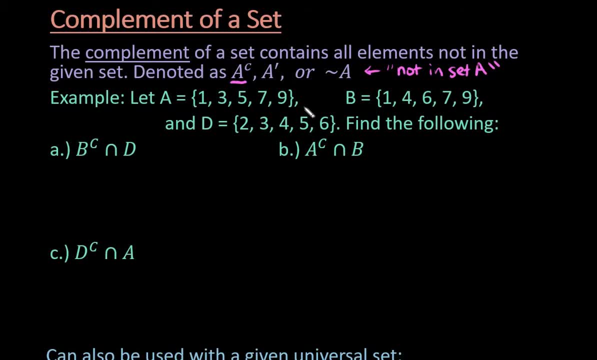 our real number system that are not in this set. So it could be a very large amount of numbers or you can narrow it down to where you're dealing with multiple sets. So I have set a as one, three, five, seven and nine. B is one, four, six, seven and nine, And D is two, three, 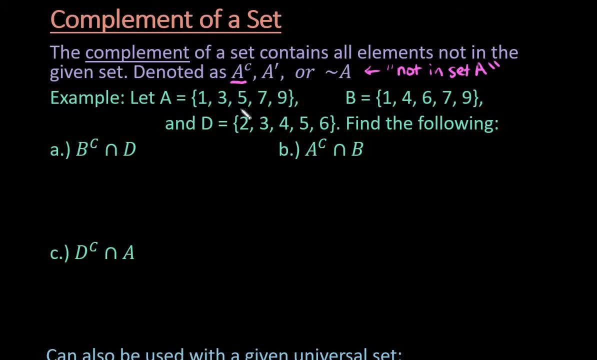 four, five and six. I chose not to use C as a set name, even though you can, just because of the symbol that I'm using, But it doesn't matter what your sets are called. Okay, so for this first one, we are looking for everything that is not in B. 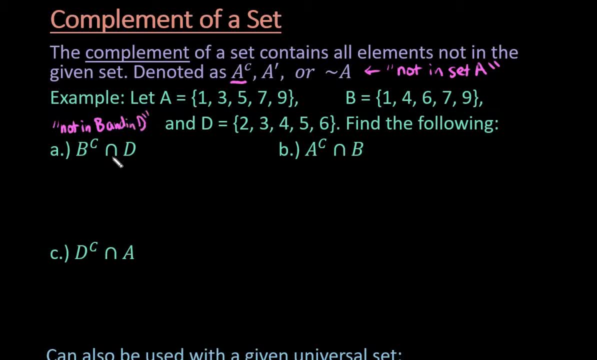 and in D. So remember that this symbol means and So basically what we're looking for here is everything that is in set D that is not also in B. So I have the numbers two, three, four, five and six. We can see that four and six are both in B, So those we would want to eliminate. So our answer. 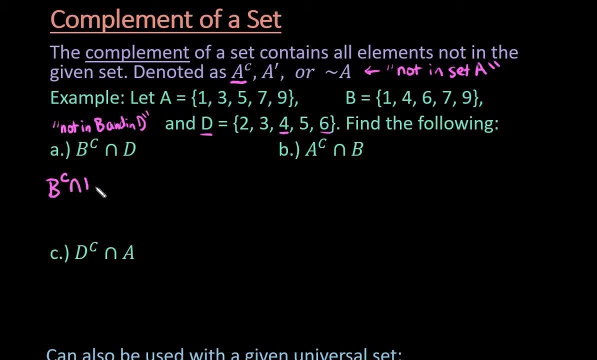 to this the not in B and in D, we would just say, are the numbers two, three and five. Okay, so, moving to the next one, we're looking for everything that is not in A but it is in B. So this time we're going to look at B and I'm going to eliminate anything that I see in A. 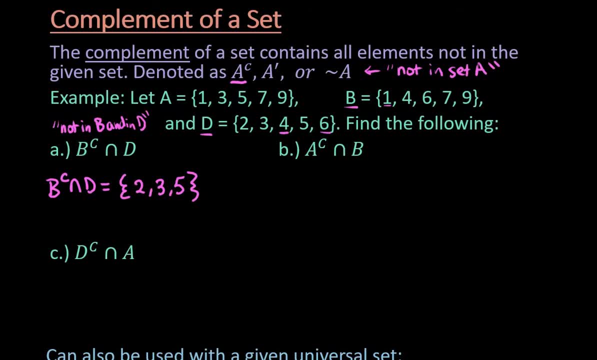 So we know that A has one in common. I tried to switch colors, All right. so we're looking at B and we know that one is in there: Four, six, seven and nine. So the only two numbers that are left that we would not eliminate for this one would just be four and six, So four. 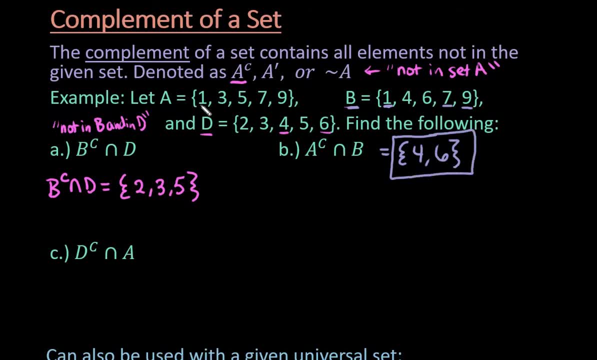 and six are the numbers that are in B and not in A. Then, for the last one that we have, we have set D, so it's not in set D and it is in A. Okay, so this time we're going to be looking at my elements in A and we're going to look at my elements in D and my elements in A. 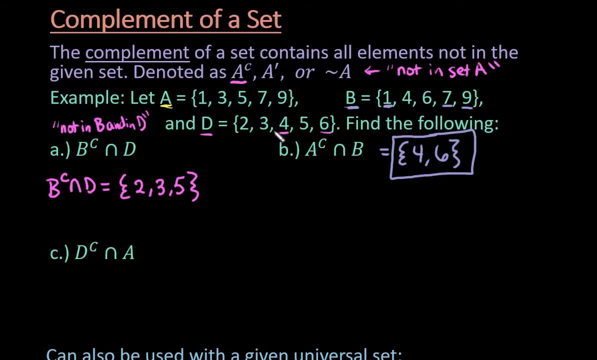 eliminate any elements that we see that are in D, because we only want things that are in A but not D. okay, so I would eliminate the three and the five. the one, seven and nine are not in D, so I can just say that this is one, seven and nine: okay. so for this one we're looking for. 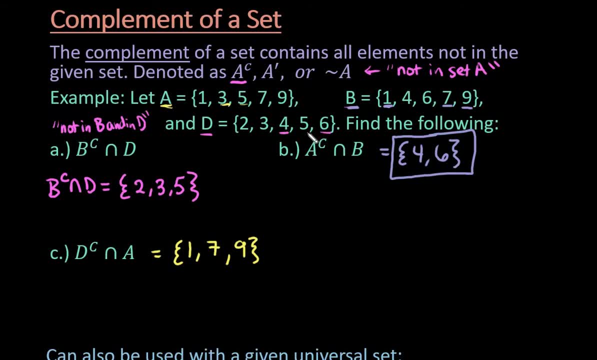 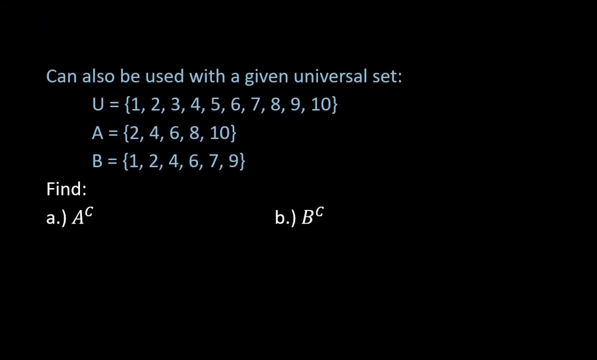 the elements that are in set A and not in D, so we eliminated everything that they have in common. a lot of times you won't see it like this in a textbook. the textbook that I'm currently teaching from does do it this way most of the time. you're going to see complement given this way, where 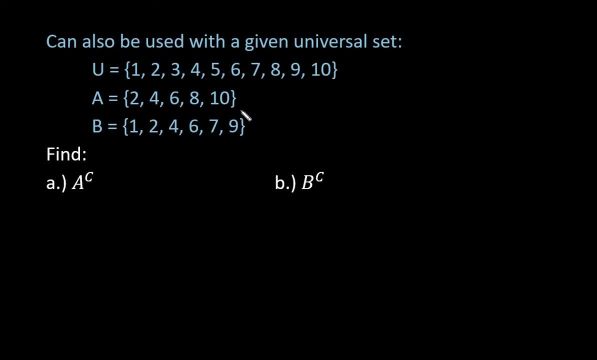 you're given a universal set and you're given values for two other sets. so this is known as the universal set whenever a U is used, and that's saying those are the only numbers that can be used for this particular problem. so for this one, our U is one, two, three, four, five, six, seven, eight, nine and ten and so. 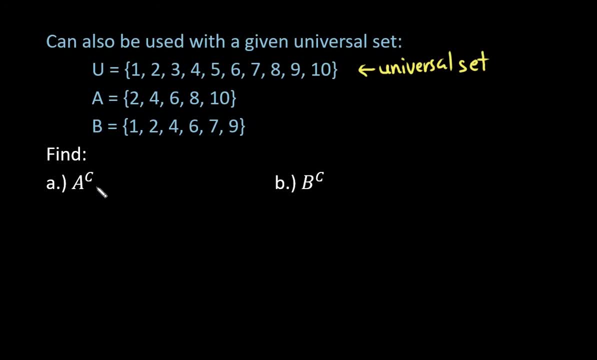 for our first example, we're looking for everything that is not in A, so your textbook could have written this as find A prime, or it could have said find tilde A, same for this one. it could have said find B prime or tilde B. so all three of these mean the same thing as far as the notation goes. so it's. 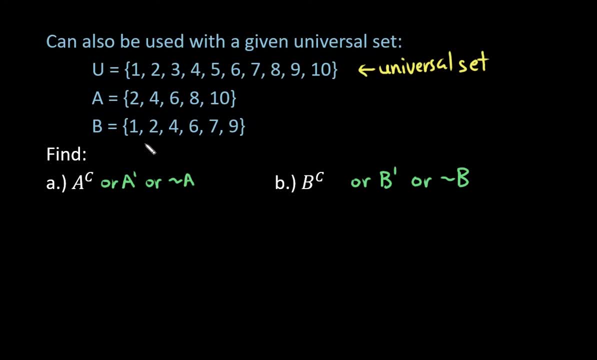 just a matter of preference of the author. I personally prefer either this one or this one, but, like I said, the book that I'm using right now uses this symbol. okay, so what we're going to do is we're looking at A, so we're looking at all of the values that are in our universal set that are not. 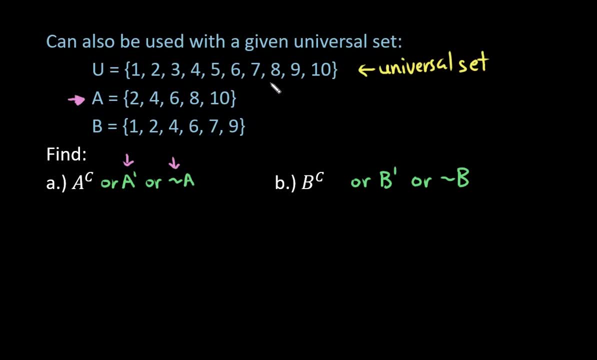 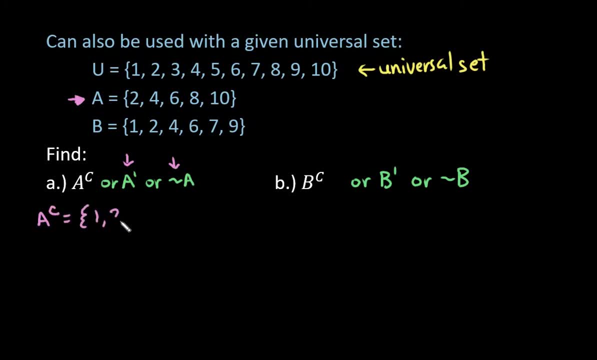 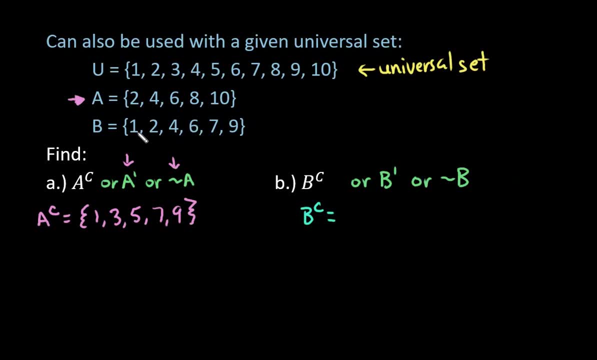 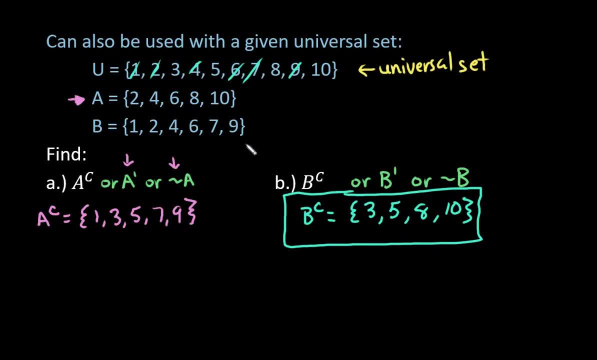